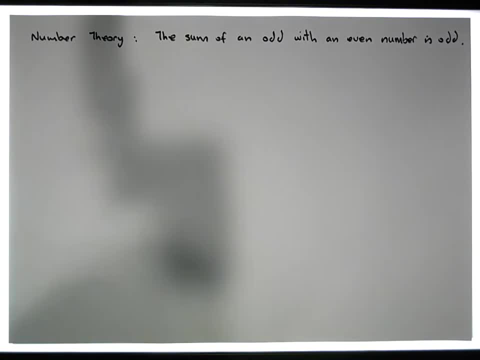 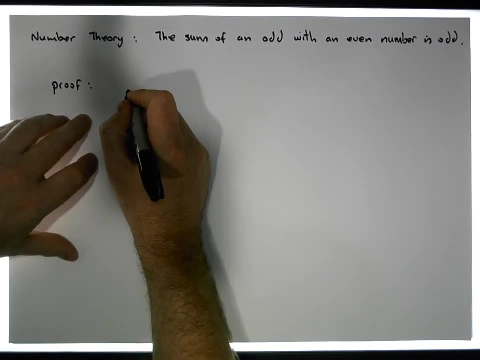 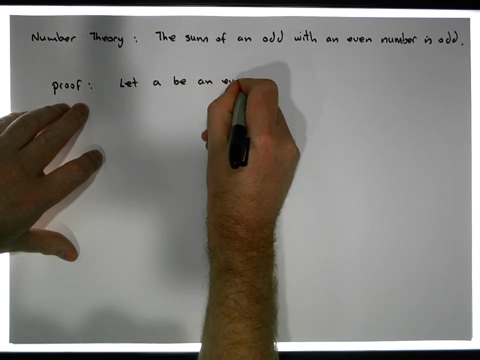 with an even number is actually, in fact, an odd number. So the proof, so our proof. So I'm just going to say: it doesn't matter which one we choose to be odd or which one we choose to be even. we're just going to say: let A be an even number, an even number, and let 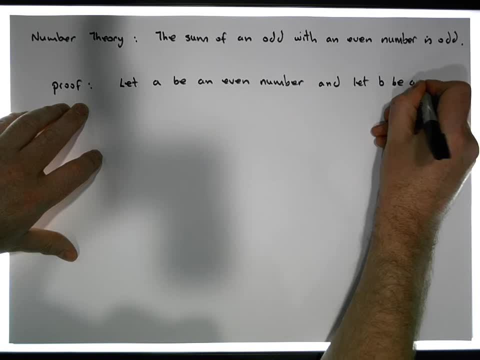 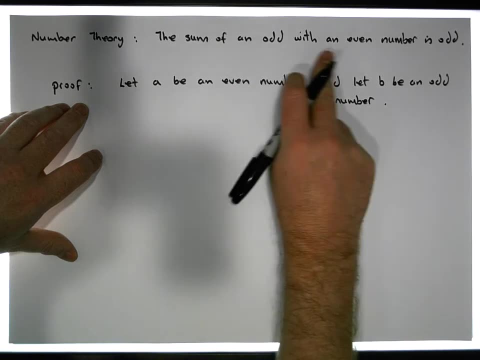 B be an odd number, an odd number. So what does this tell us about A and B? Because we can't actually show that the sum of an odd and an even number is odd unless we actually have an odd number and an even number. So 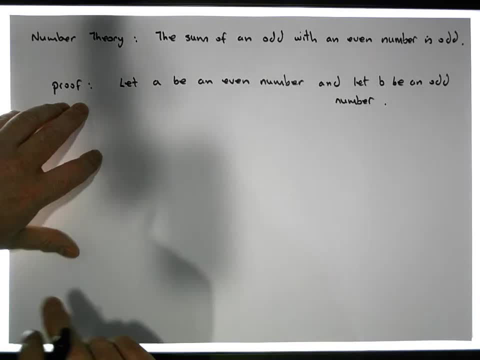 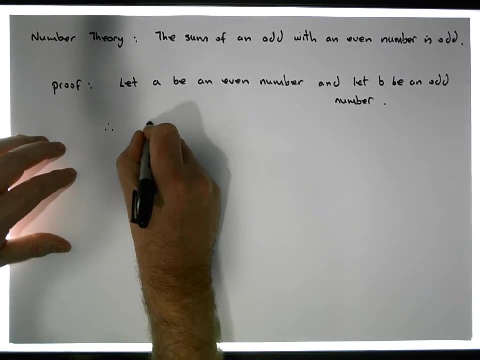 we're just going to assume that A is an even number and that B is an odd number. What does that tell us about them two numbers? Well, that tells us that A, well, A, is even. so A must be able, we must be able to write A in the form of A is equal to two times some other. 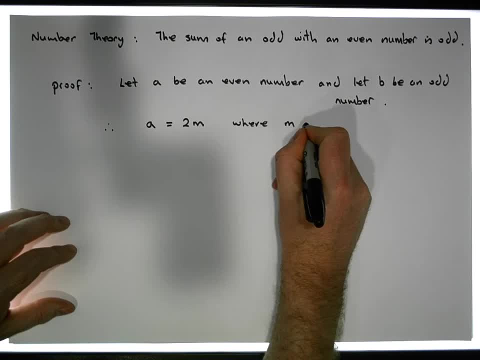 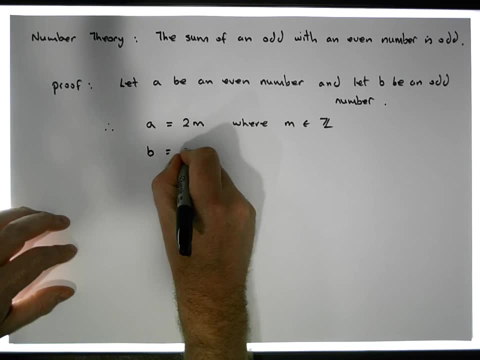 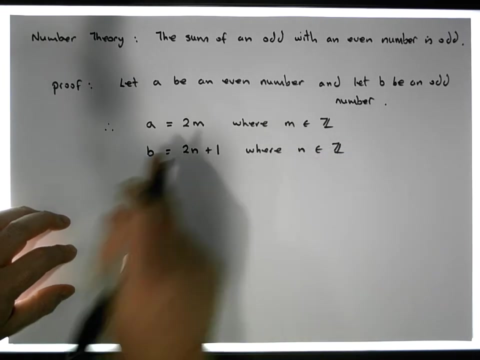 number. okay, where M is an element of the integers- And we get that from the division algorithm, And also B being an odd number. well, B must be equal to two times some other number, plus one where N is an integer, And this comes once again from the division algorithm. 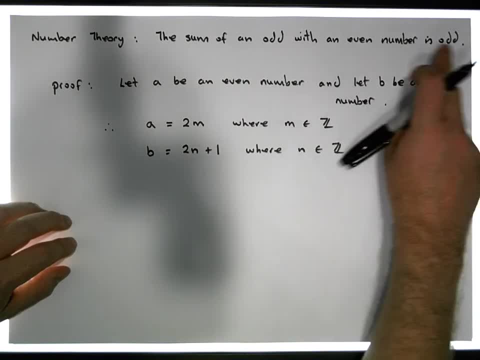 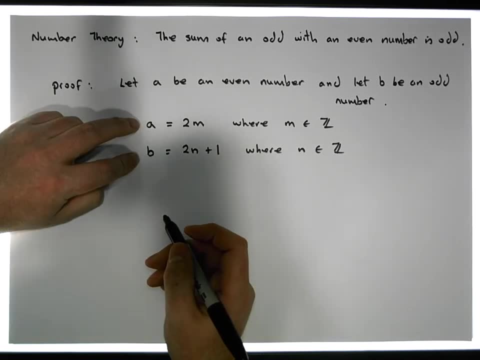 So what we'd like to show is: we'd like to show that the sum of an odd number with an even number is, in fact, odd. okay, Now, what we're going to do is we're just going to add A with B, but we know that the addition 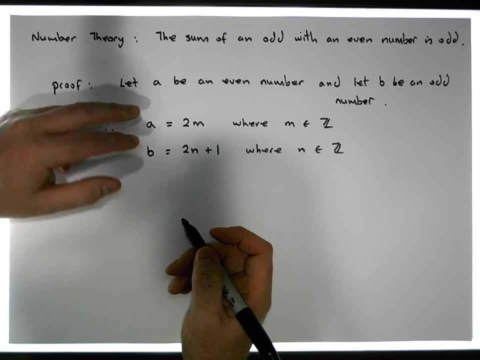 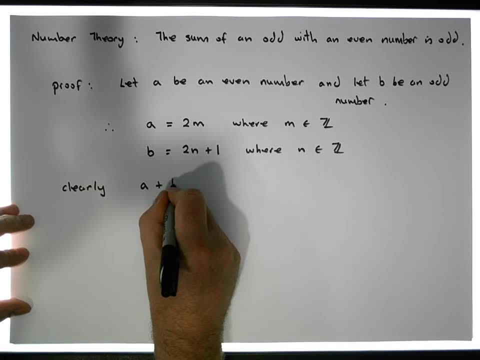 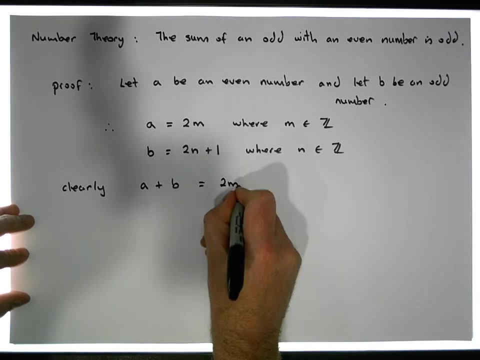 is commutative in the integers. okay, so A with B is the same as B with A. okay, So clearly we have A plus B, okay, which is the same as B plus A. okay is equal to A is 2M, okay. 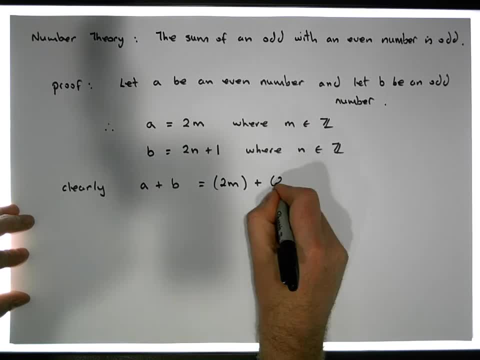 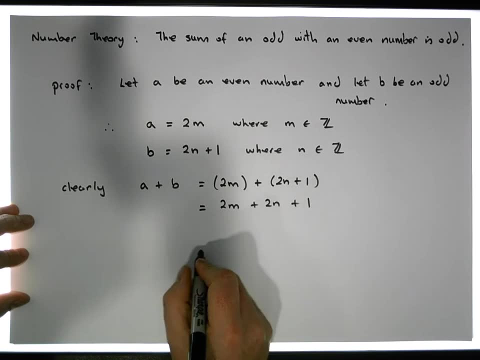 okay, plus B, by definition, which we're saying is equal to 2M plus 1.. Let's remove the brackets. What do we get? We get 2M plus 2N plus 1. There's a common two across these two particular. 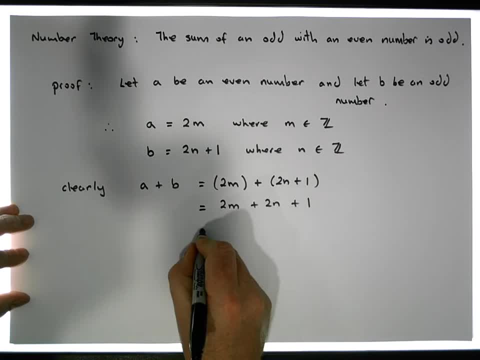 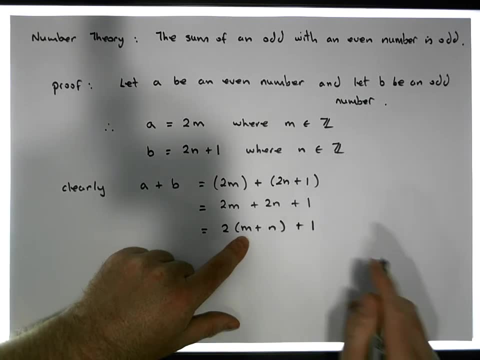 these two particular terms here. so this is equal to two times delta N. okay, Now it's going to reason B over the 16 and 17.. m plus n plus one: now m and n are integers. okay, so then that means that m plus n is an element.